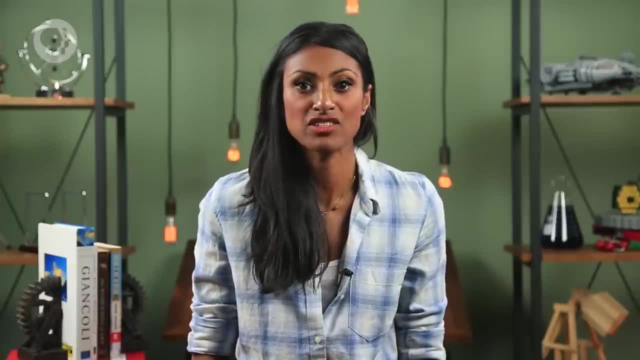 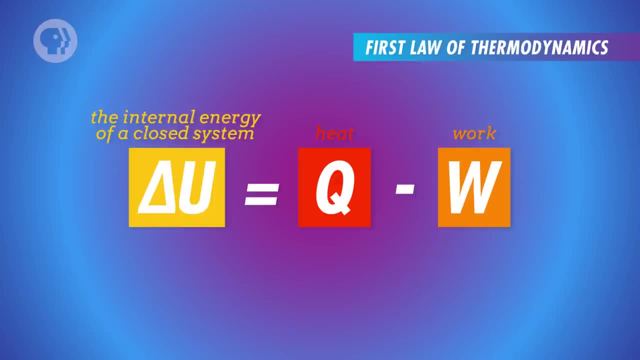 So we can have an equation to use for analyzing problems. We write the first law like this: The internal energy U of a closed system is equal to Q, Q the heat transferred to the system, minus W the work done on or by the system. 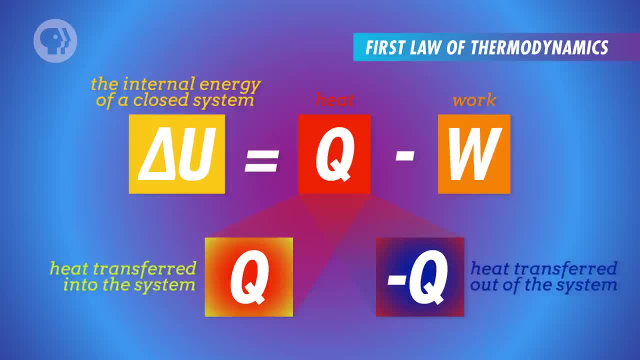 It's important to remember that when we talk about changes in internal energy, if heat is transferred into the system Q is positive and if heat is transferred out of the system Q is negative, And if work is done on the system W is negative and if work is done by the system W is positive. 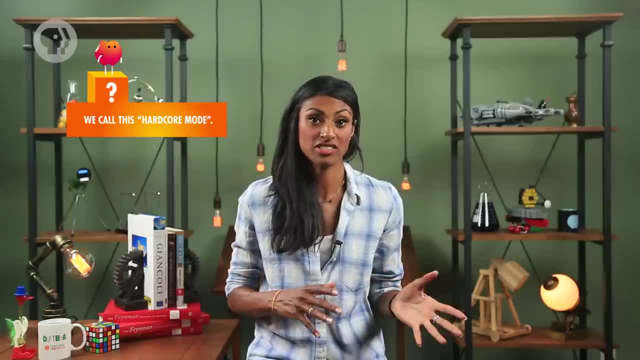 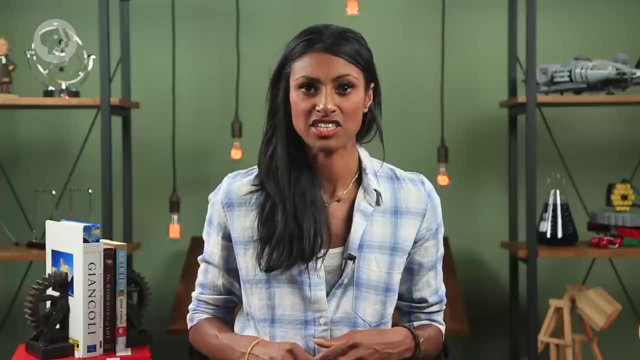 Some textbooks will change those signs around, so it's worth keeping track of what the positives and negatives mean. Now you'll notice that the first law of thermodynamics describes only those two factors- work and heat- As affecting a change in internal energy. That's because, as long as the system is closed, meaning it's isolated from the rest of the universe, there just aren't any other factors involved. The amount of heat lost by the system is exactly equal to the amount of work done by the system, and vice versa. 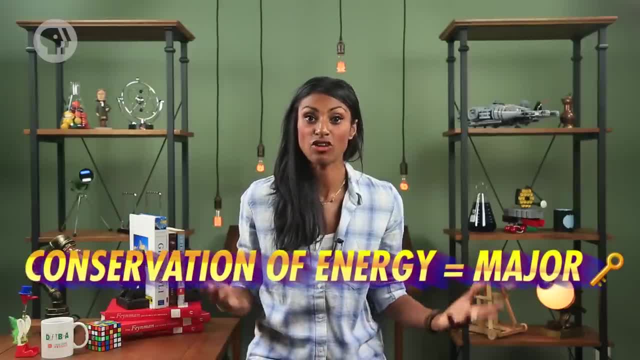 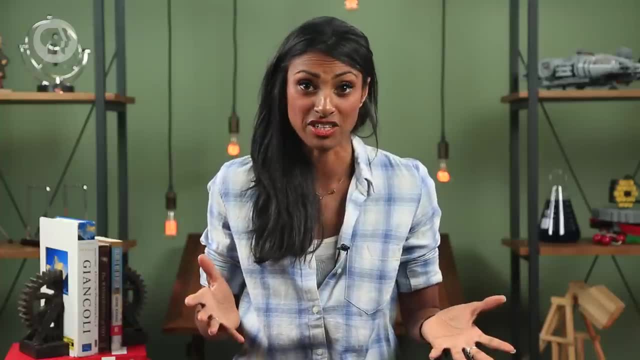 So really, the first law of thermodynamics is just another way to describe the conservation of energy which keeps coming up in our lessons, because it's such a key principle of physics. There's always some kind of heat loss, like through friction. Even that tiny amount means that the motion can't continue forever. It will eventually run out of the energy it needs to drive the work it's doing. That's part of why the drinking bird isn't a perpetual motion machine. It relies on the energy it gets from the cup of water to power its movement. The bird is filled with a fluid that has a low boiling point, so it can easily change from a gas to a liquid and back, with just a slight change in temperature. 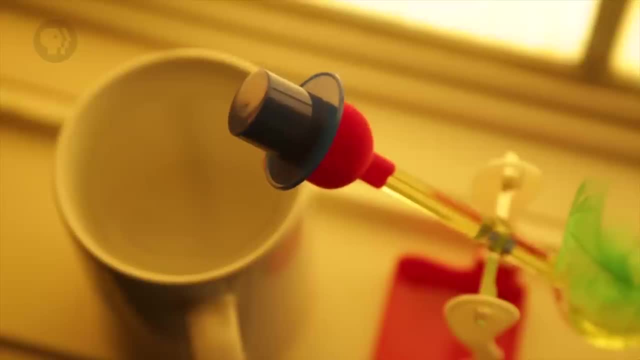 There's some liquid at the bottom and some vapor at the top. When the bird's head dips into the cup, it gets wet, It keeps bobbing back and forth for a while and as the water evaporates it cools the vapor in the bird's head. 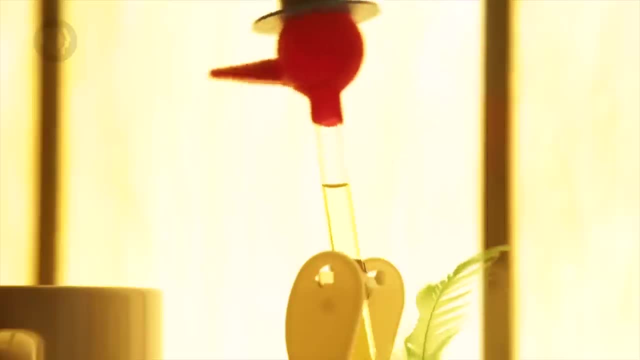 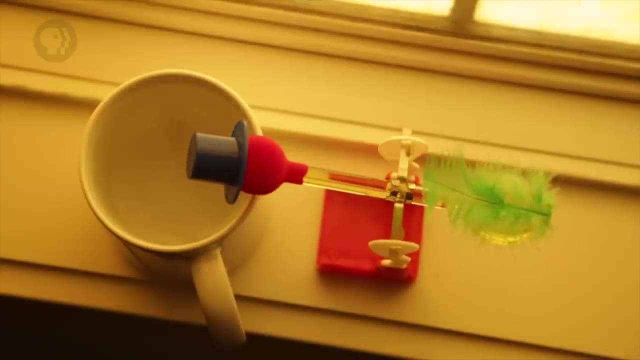 which condenses into water. Then it goes into liquid, creating a partial vacuum in the head. That makes liquid travel up the tube. The head gets heavier and dips back into the water, But the tipping makes a bubble rise through the liquid into the bird's head, sending more liquid into the bottom. 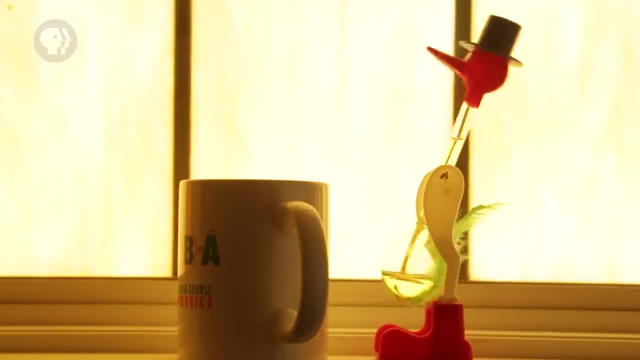 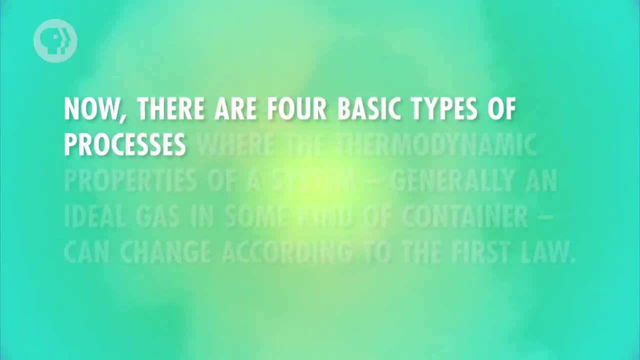 and setting the little bird swinging and starting the cycle all over again, But it still needs the water for it to do its thing. Once the water in the cup runs out, the bird stops moving. Now there are four basic types of processes where the thermodynamic properties of a system – 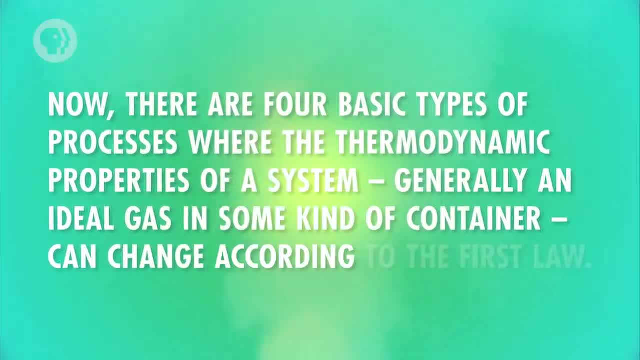 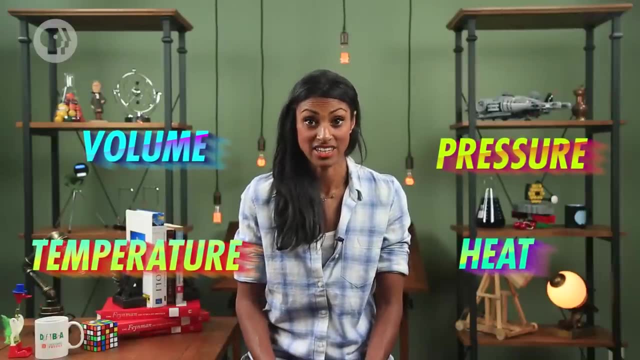 generally an ideal gas in some kind of container – can change according to the first law. In each case, one property is held constant – volume, pressure, temperature or heat – while the other properties change. Variations on all these properties are used in all kinds of machines, especially engines. 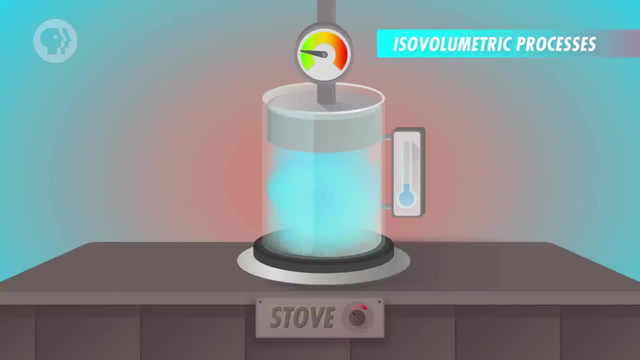 First, there are isovolumetric processes where the volume is held constant, usually because the gas is in a rigid container while heat is added or removed. As you add heat, the pressure of the gas will increase and so will its temperature. 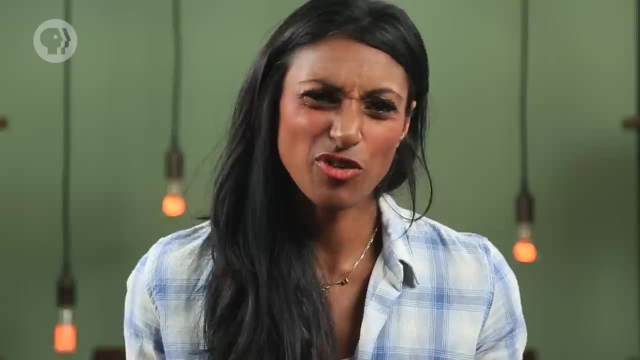 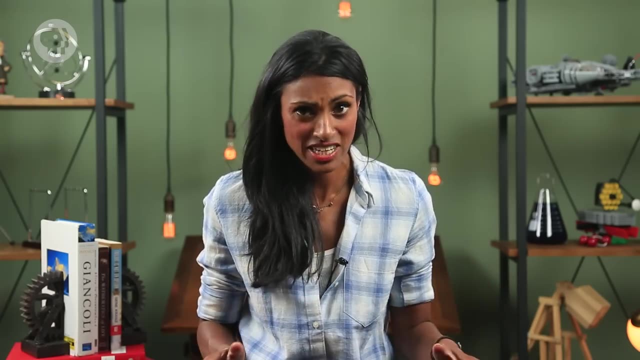 As you remove heat, the pressure and temperature will decrease. Isovolumetric processes are kind of boring. As thermodynamic processes go, the gas is stuck inside its container and no matter how much heat you add, the gas doesn't do any work – you're just increasing its internal energy. 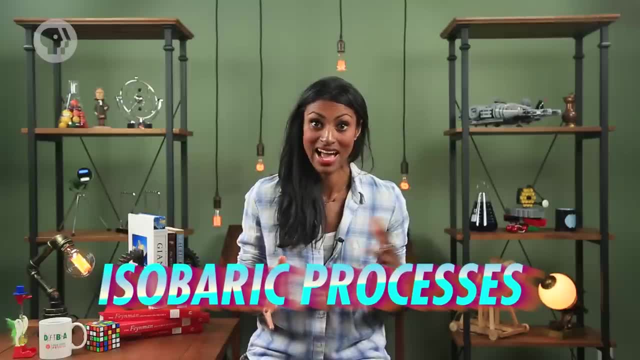 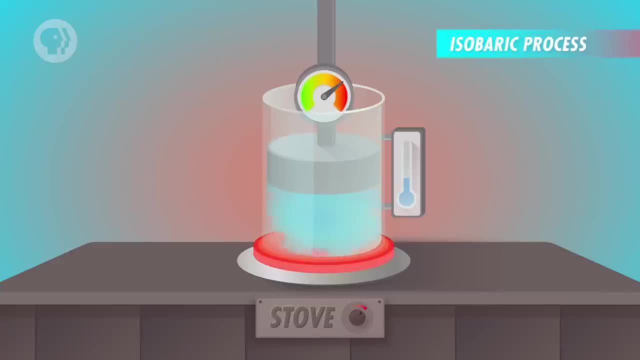 But isobaric processes, where the pressure is held constant while heat is added or removed, are a little more interesting. Here the volume of the container is allowed to change, usually because the gas can move a piston. As you add heat, the volume and temperature of the system increase, and as you remove heat, the volume and temperature decrease. 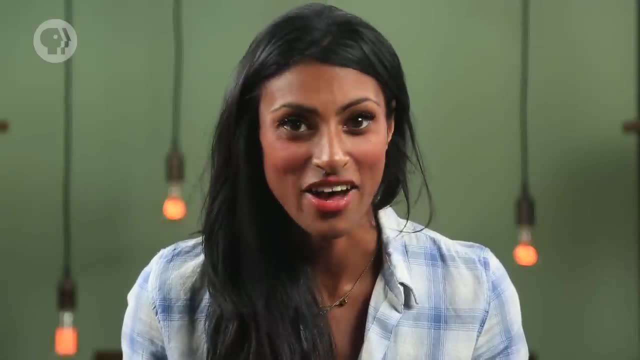 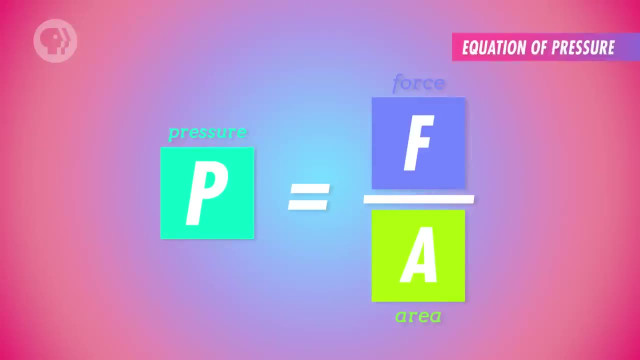 Which means that an isobaric process can do work. Here's why, In earlier episodes we've said that work is equal to force times distance – in this case the distance the piston moves. We've also said that pressure is equal to force divided by area, which means that force is equal to pressure times area. 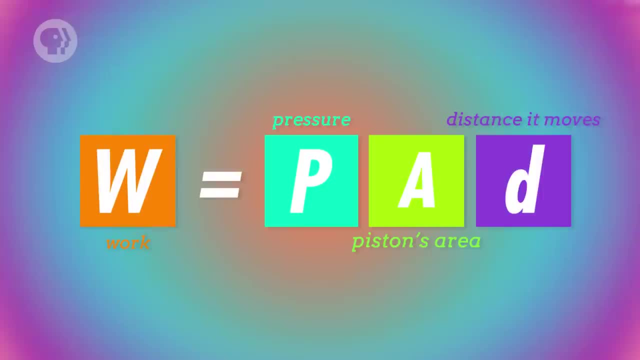 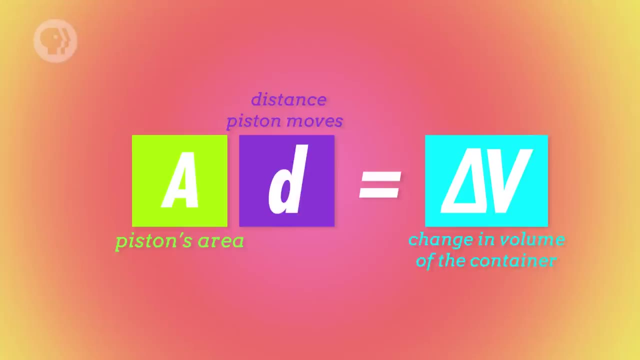 Here is the pressure of the gas times the area of the piston. So work is equal to the gas's pressure times the piston's area times the distance it moves. And one more step – the area of the piston times the distance it moves will be equal to the change in the volume of the container. 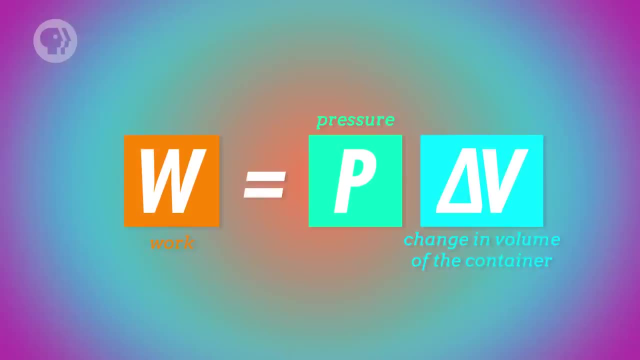 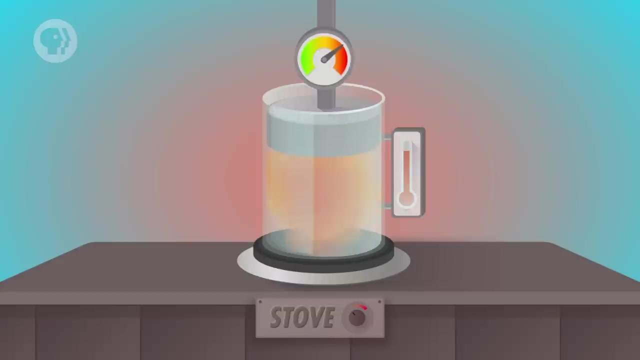 So the work done during an isobaric process is equal to to the pressure of the gas times the change in the volume. If heat is added, the volume goes up and the piston moves outward. so the system does work. If you push the piston inward, you're doing work on the system, so its volume goes down. 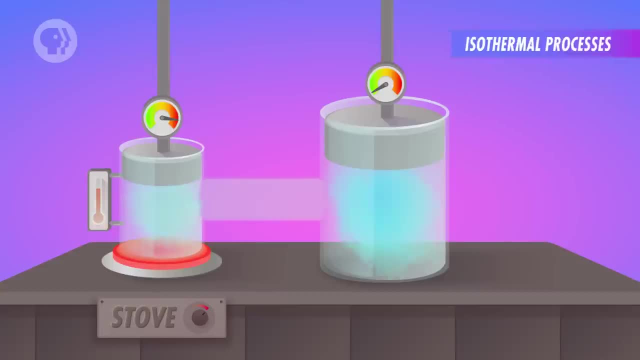 The third type of thermodynamic processes are isothermal, That's where temperature is held constant, usually by connecting the system to a much bigger system whose temperature would take a lot of heat to change, known as a heat reservoir. The heat or volume of a system is then changed very slowly so that the other properties 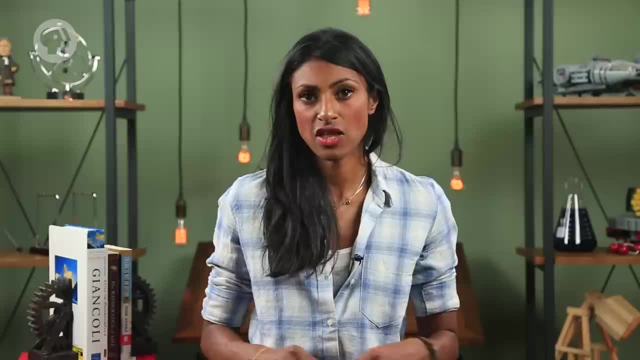 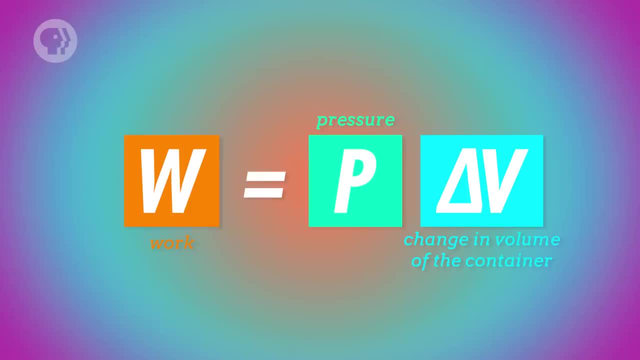 can adjust, while the temperature essentially stays constant. An isothermal process is kind of like an isobaric process, in that if you add heat the volume will expand, so the system will do work. But for isothermal processes you can't use that simple W equals P, delta V equation. 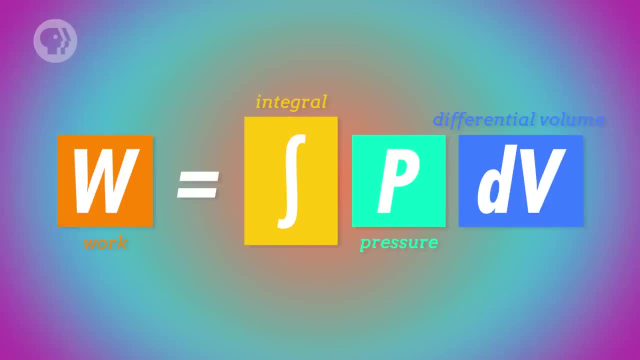 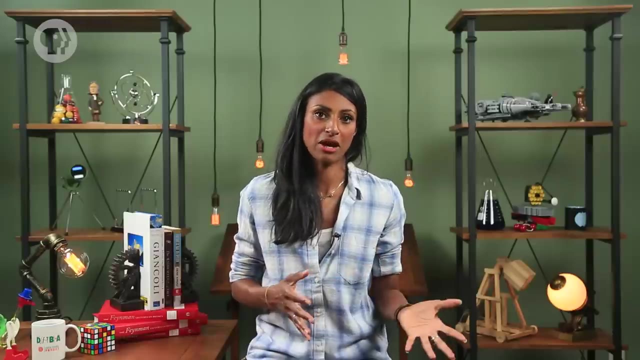 because the pressure does change. Instead, you need to take the integral of the pressure with respect to volume. This way, you're still calculating work, but you're taking the changes in pressure into account too. Another difference between isobaric and isothermal processes is that, since temperature is held, 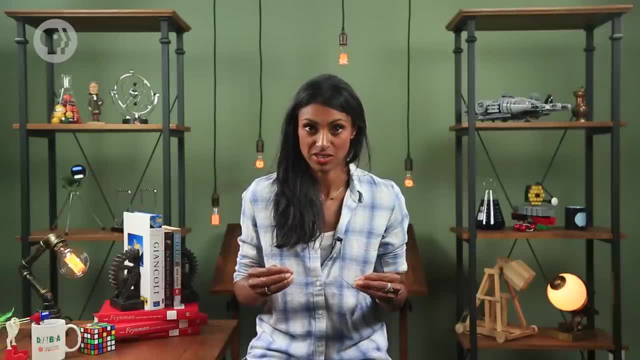 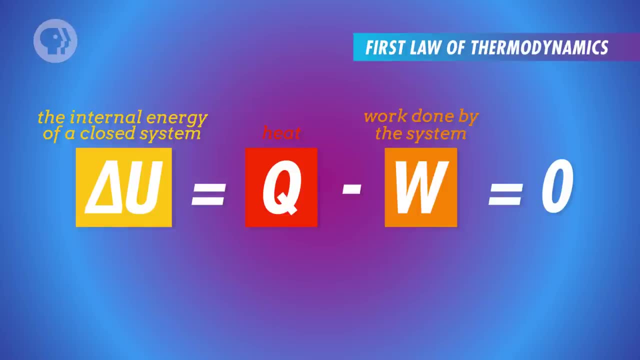 constant. in isobarics it's not always constant. In the case of isothermal processes, the internal energy of the ideal gas can't change And the first law of thermodynamics says that heat minus work is equal to the change in the internal energy of the system, in this case zero. 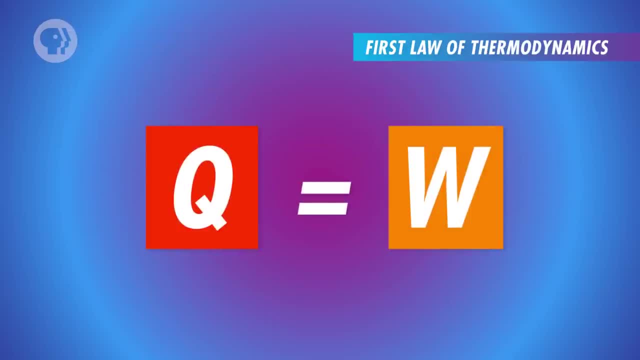 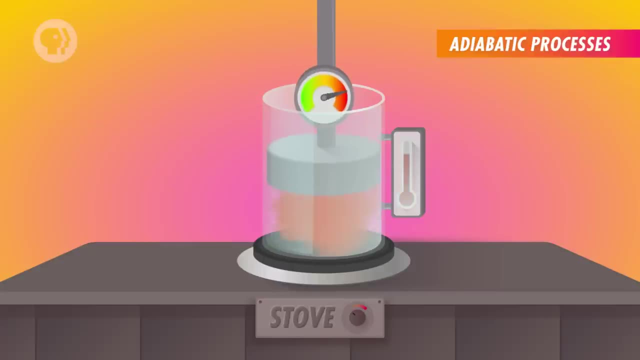 So the work done by the system will be equal to the amount of heat added, and vice versa. Finally, there are adiabatic processes, where no heat is allowed to flow in or out of the system, but the gas can expand or be compressed. 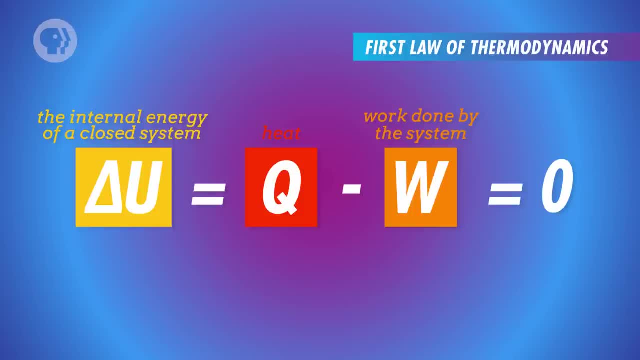 Again, the equation for the first law of thermodynamics helps us out here. Q is zero because the heat of the system isn't changing, But the internal energy of the gas can change. so the system can do work or have work done on it. 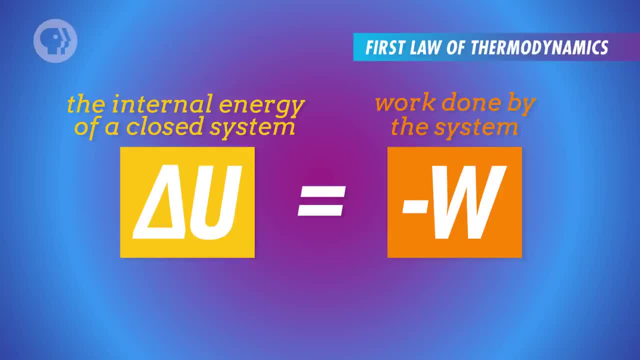 In fact, the change in the internal energy of the gas will be exactly equal to the negative of the work. But this is all just the first law of thermodynamics. There's also the second law, which says that heat will spontaneously flow from something. 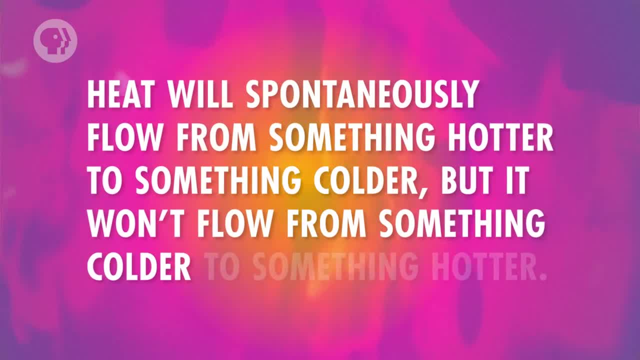 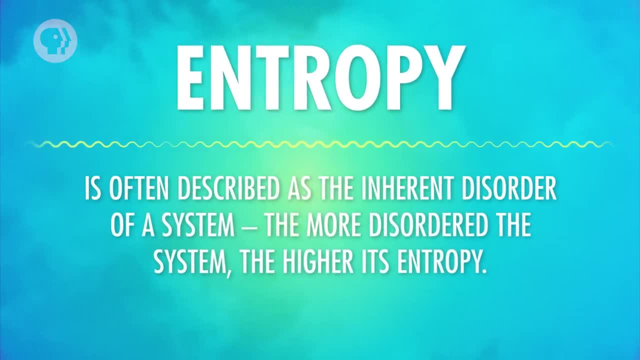 hotter to something colder, but it won't flow from something colder to something hotter, And that's because of this thing called entropy. Entropy is often described as the inherent disorder of a system. The more disordered the system, the higher its entropy. 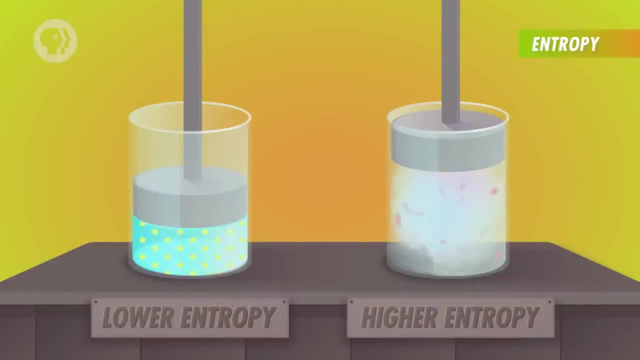 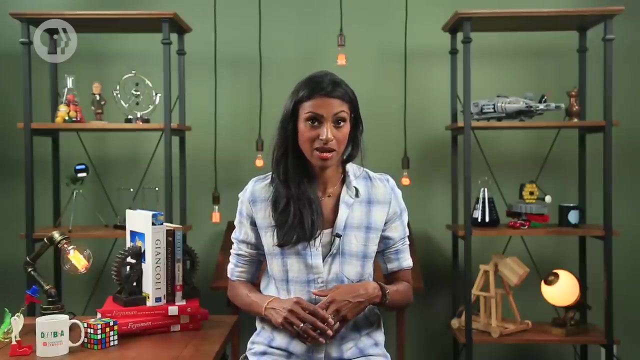 So a gas, for example, is a gas that's hot. It's not hot, But a molecule with all its molecules randomly bouncing around has a higher entropy than a solid with its molecules neatly arranged. And a more general way to state the second law of thermodynamics is that in real life, 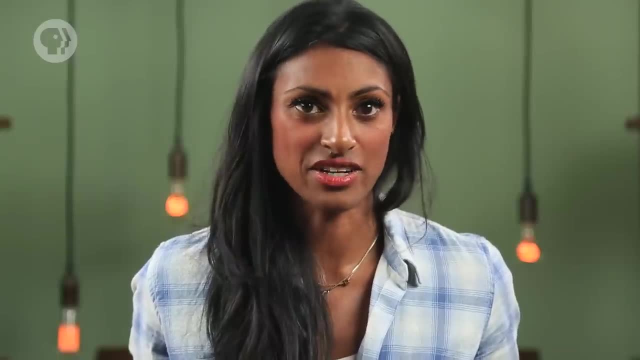 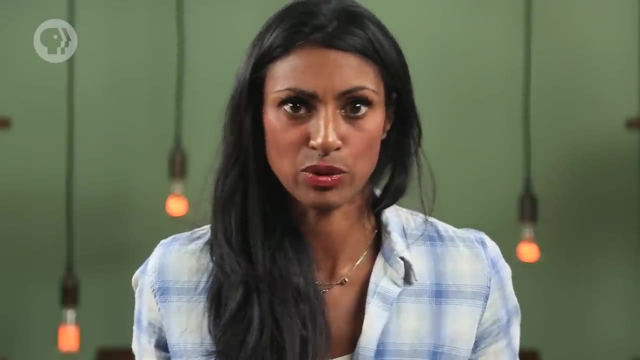 entropy can only increase overall. That doesn't mean that entropy can never decrease. in certain situations, Like gases do sometimes turn into liquids or solids. obviously You've seen water vapor condense and liquid water freeze. But if the entropy in a system decreases, that means the entropy of the environment. 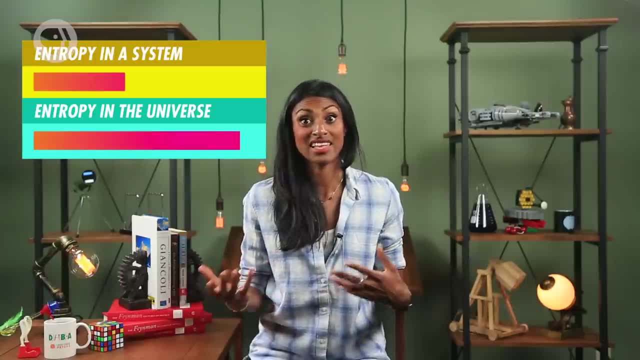 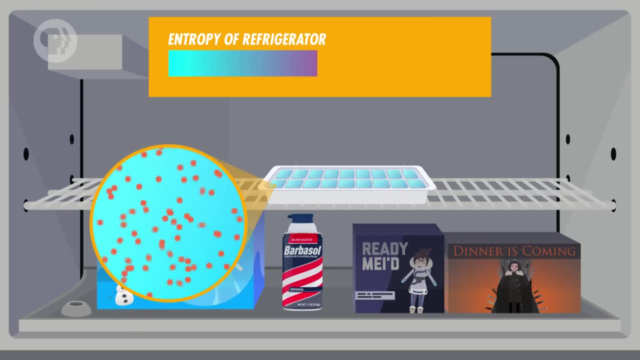 around the system must increase enough to compensate, and then some So that there's an overall increase in the entropy of the universe. Say, you put water in your freezer to make ice, for example, The entropy of the water goes down as it freezes. 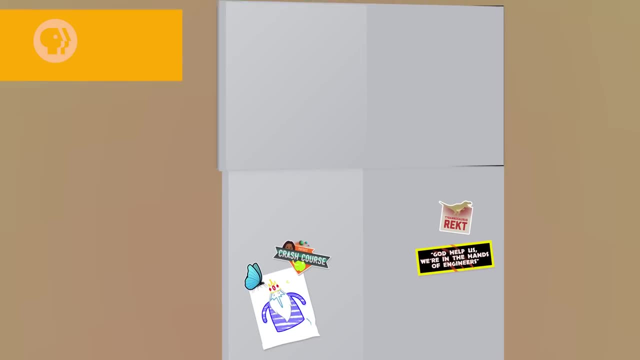 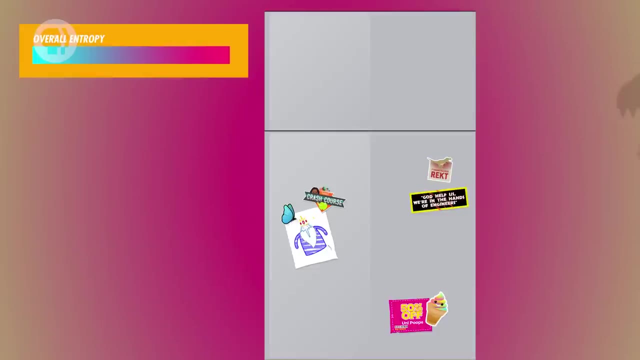 But meanwhile your freezer is putting out heat as it works to keep itself cold inside, And the heat from your freezer is increasing the entropy of your kitchen more than the entropy of the ice is decreasing, So overall there's an increase in the entropy of the universe. 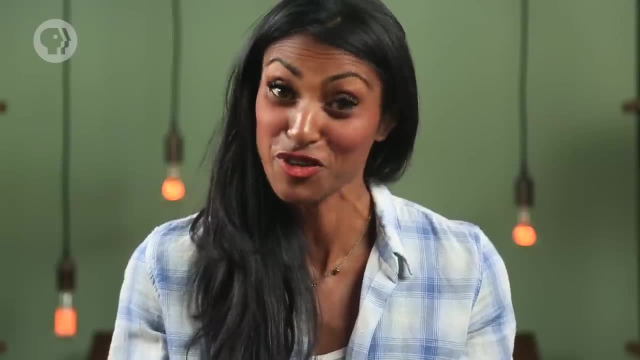 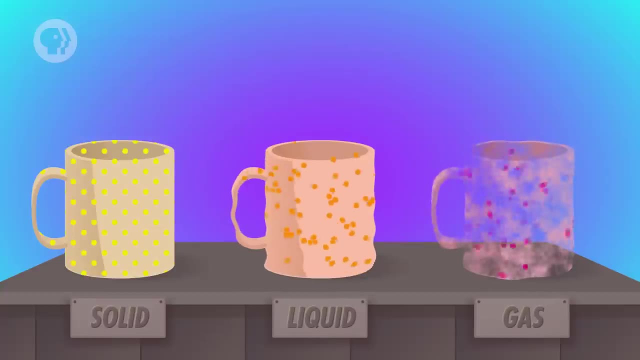 Remember that Every time you're making ice, you're increasing the disorder of the universe. Now, entropy's tendency to increase has to do with probability. To see what I mean, picture a shape. Picture a shattered ceramic mug. There are molecules that make up that mug and there are lots and lots of ways that those 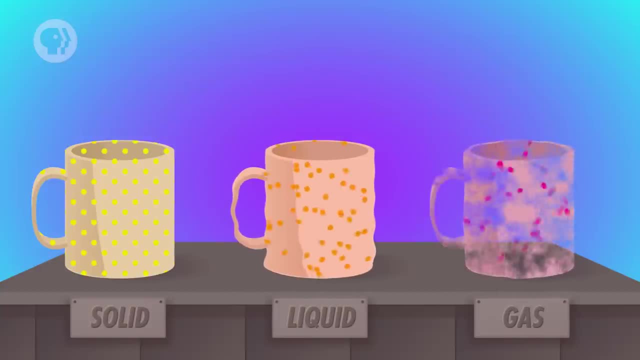 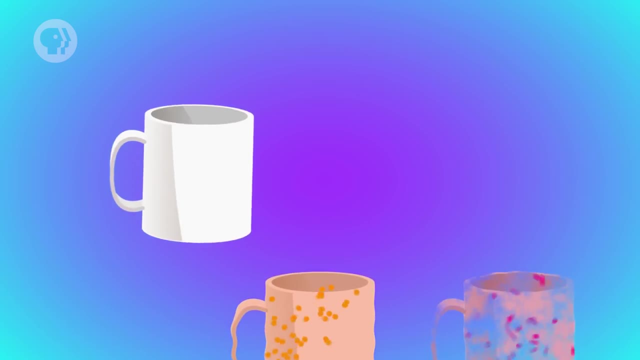 molecules can be arranged in space and all of them are equally likely, But only in a few of those arrangements can the molecules make up a whole solid, unshattered cup – the state where they have a lower entropy. Still there are lots of possible arrangements of those molecules where they could make up 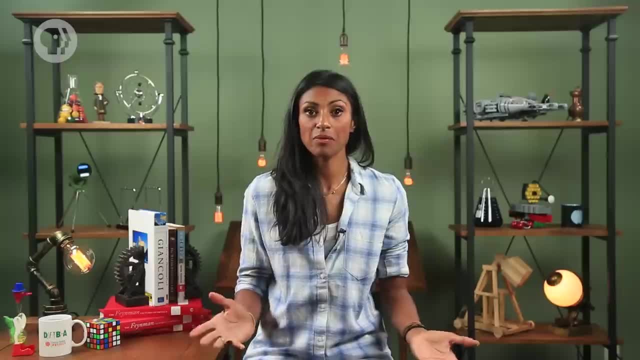 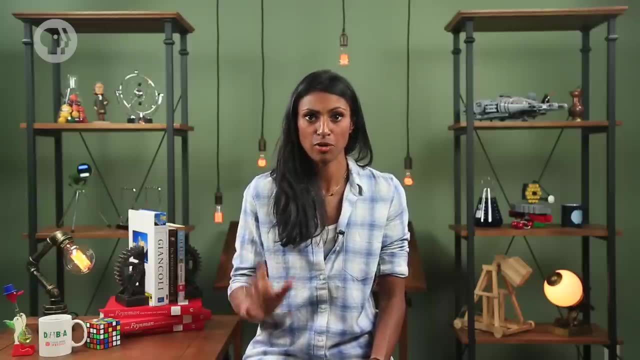 a shattered cup – a set of pieces with a higher entropy. The cup can be shattered into pieces – 300 pieces, with the pieces far apart or very close together, And every way the cup can shatter is another possible way for the molecules inside the. 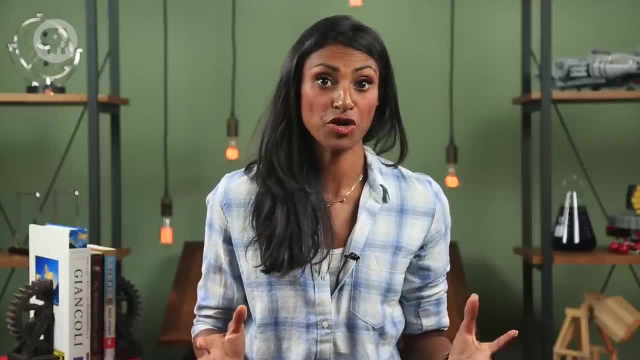 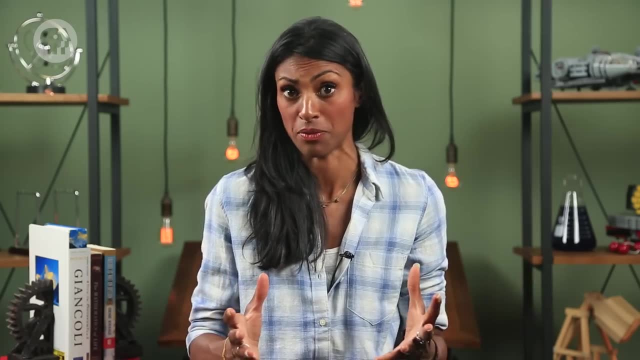 pieces to be arranged. But when there are so many ways for the cup to be broken and so few ways for it to be whole, it becomes very, very unlikely that the pieces will spontaneously put themselves back together if you drop them. Basically it'll never happen. 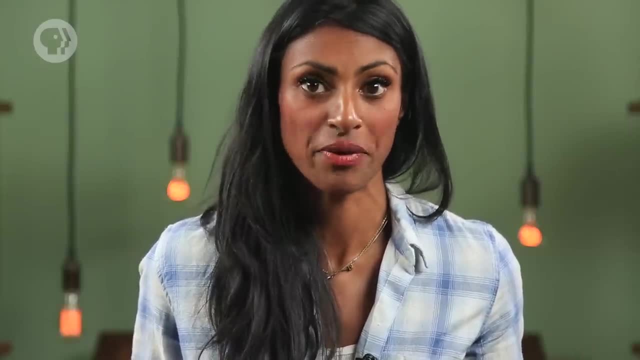 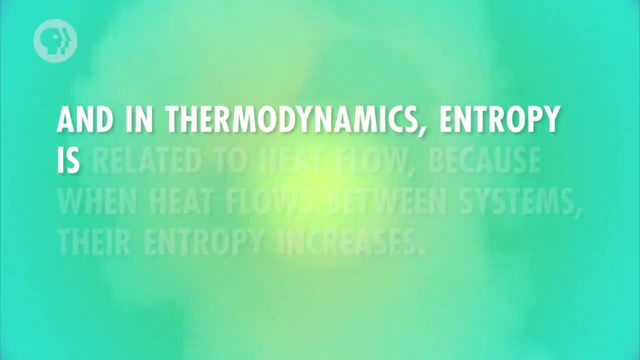 On the other hand, it's very likely that a cup that's whole will break when you drop it. So the process that leads to an increase in entropy has a much higher probability of happening. And in thermodynamics, entropy is related to heat flow, because when heat flows between 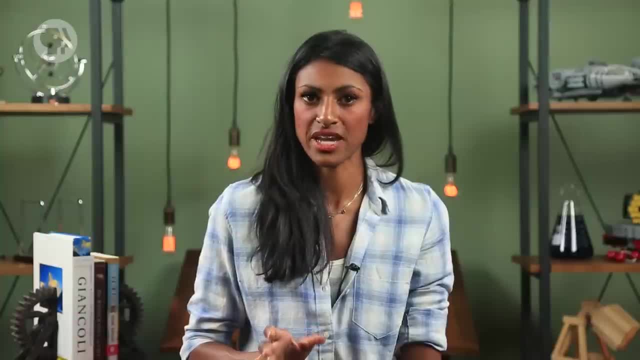 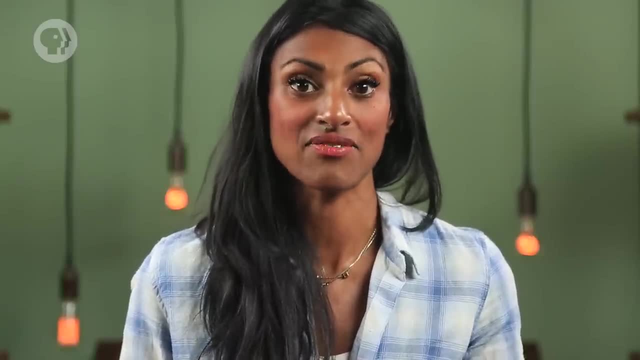 systems, their entropy increases. Before, when their molecules were different temperatures, that was an orderly arrangement. But when their temperatures become equal, that neat organization is gone. so the systems have a higher entropy. So heat spontaneously flows from warmer systems to cooler ones, because that leads to an increase. 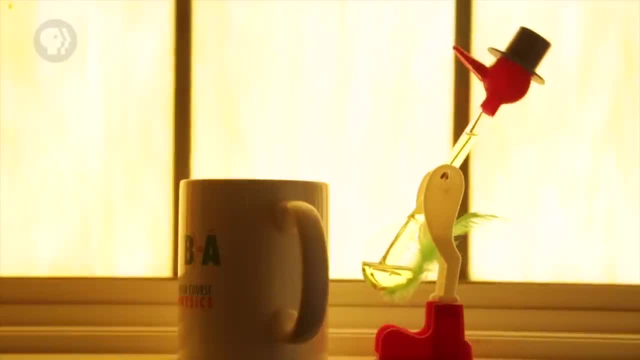 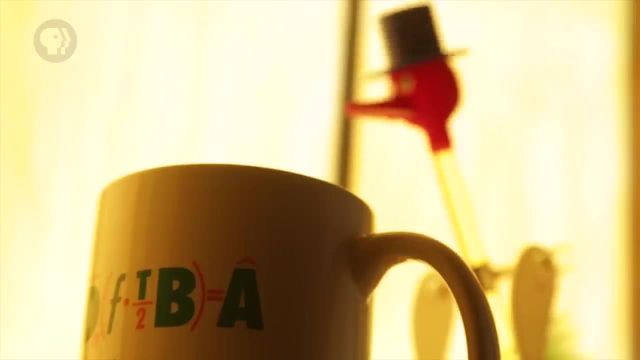 in entropy, Which is also why this little bird keeps bopping up and down. When the heat flows out of it, the gas condenses and it dunks into the water. The bird may not be a perpetual motion machine, but it's a great way to see the first and 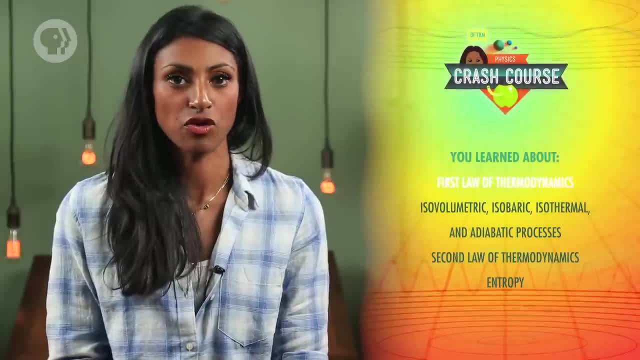 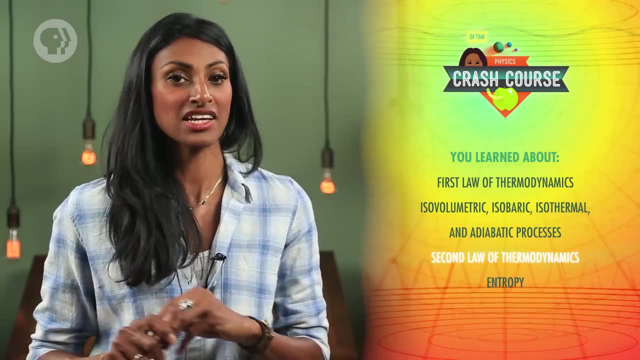 second laws of thermodynamics in action. Today you learned about the first law of thermodynamics and how it applies to isovolumetric, isobaric, isothermal and adiabatic processes. We also talked about the second law of thermodynamics and entropy. 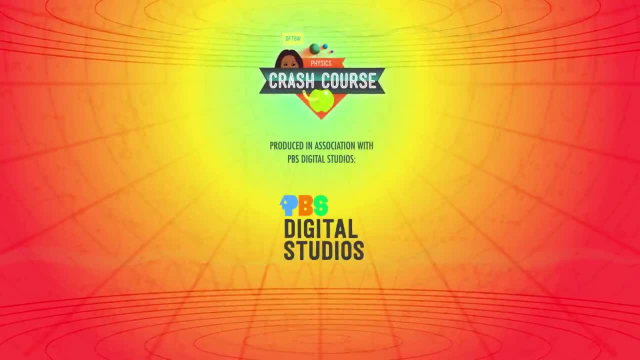 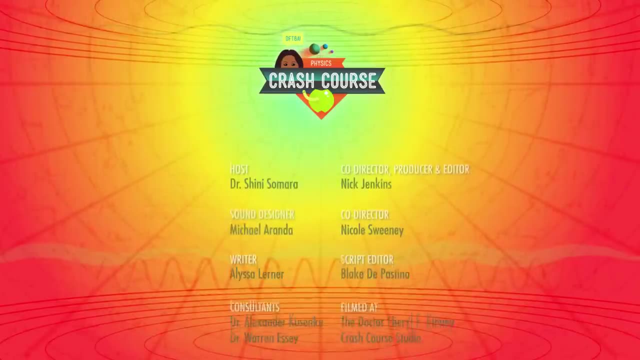 Crash Course Physics is produced in association with PBS Digital Studios. You can head over to their channel and check out a playlist of the latest episodes from shows like The Good Stuff, BrainCraft and Physics Girl. This episode of Crash Course was filmed in the Dr Cheryl C Kinney Crash Course Studio. 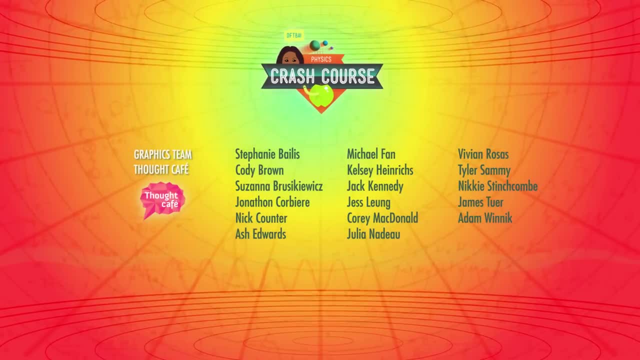 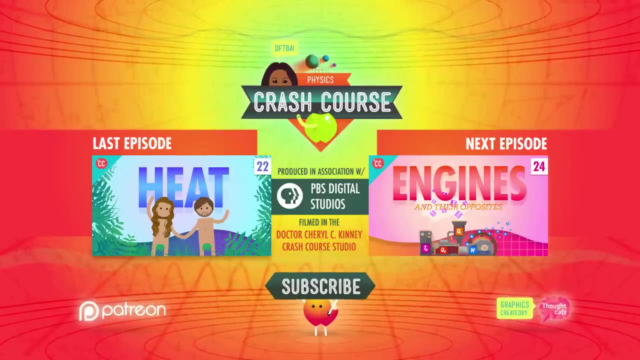 with the help of these amazing people and our equally amazing graphics team is Thought Cafe. We'll see you next time.